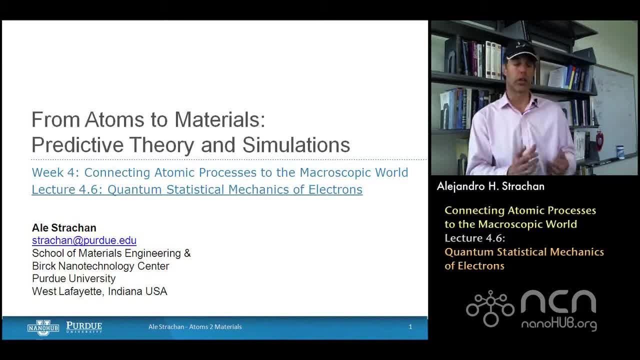 there I can put as many as I want. So in the example that we worked on, if I have a vibration of a frequency omega, I can have as many excitations of that vibration as I want. I can have zero. then the oscillator is in. 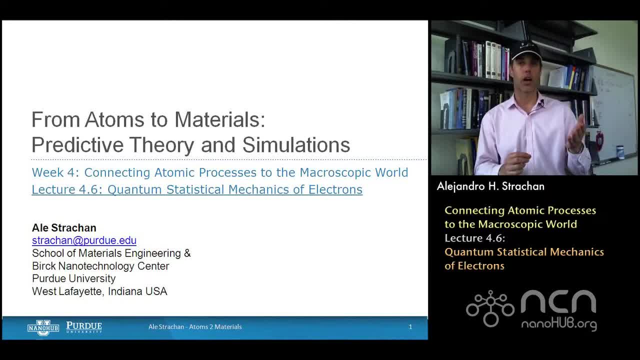 the zero has the zero point energy. one half h bar omega. I can have one excitations, two, three, four, and what that means is higher and higher energy. in that specific vibration, Electrons are completely different, because I can either have zero electrons. 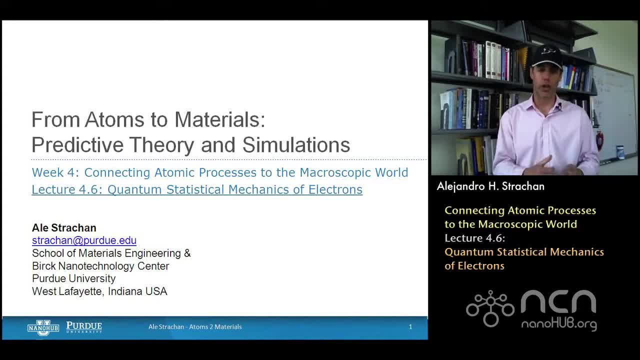 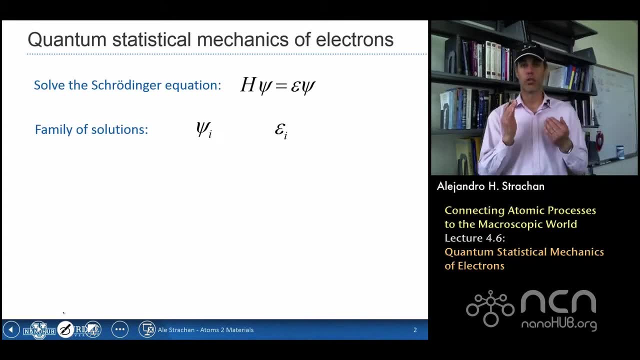 or one electron in that specific vibration. I can have one electron per state. So we're going to derive their quantum statistical mechanics. We're going to start with the Hamiltonian and the Schrodinger equation. If we solve the Schrodinger equation we get a family of wave functions. 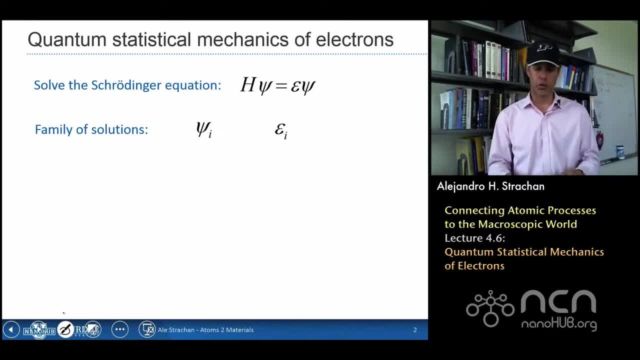 and energies, And today I'm going to use for this lecture epsilon as the eigenvalues of the energies, the energy of a particular state, And I hope you forgive me the slight misinterpretation of the energy of a particular state. I'm going to use a slight inconsistency. 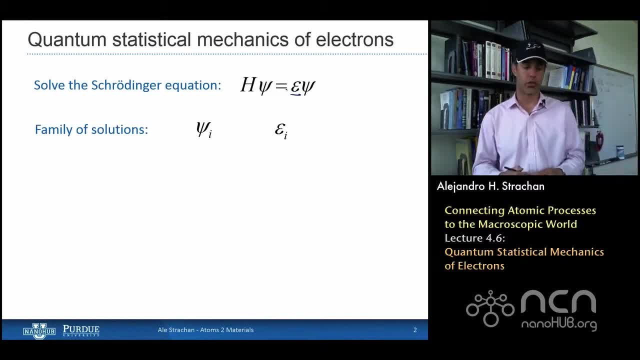 nomenclature, but I want to reserve E for the total energy of a many electron system. Alright, so I have these eigenvalues and I want to put: I'm going to consider a set of n non-interacting electrons living in these states. This is called a free. 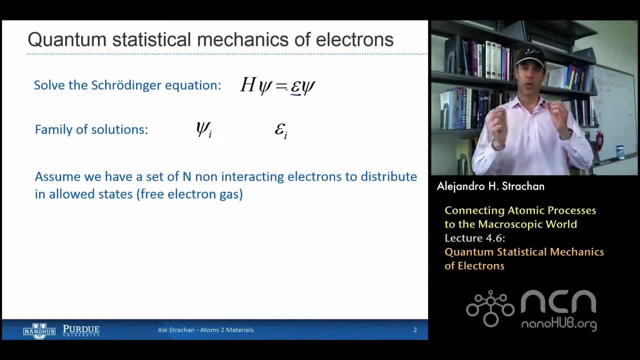 electron gas where electrons do not interact with one another. So I'm going to put a free electron gas where electrons do not interact with one another. So we know that at zero temperature the electrons are going to organize themselves in a way that they 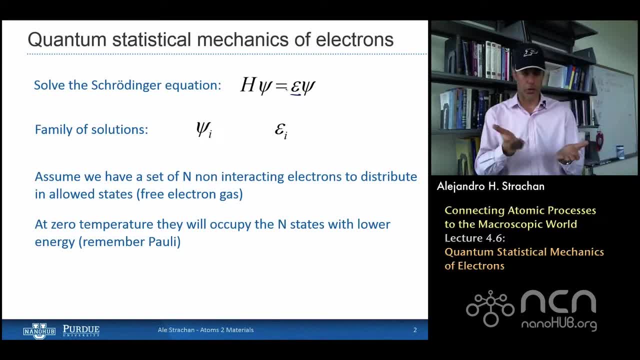 occupy the n lowest energy states. Okay, I start from the bottom and I fill them up, fill the available states up with electrons until I run out of electrons. And this is again a manifestation of the Pauli exclusion principle that does not allow me to put. 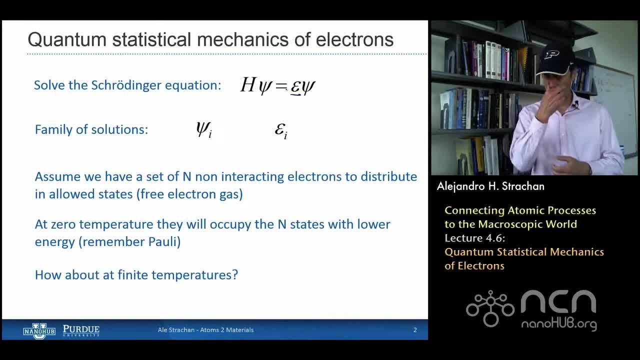 in more than one electron per state. Now the question we're going to address today is what happens with this population of electrons at finite temperatures. Okay, I can imagine that if I have a high temperature, some of the electrons may be promoted to an excited 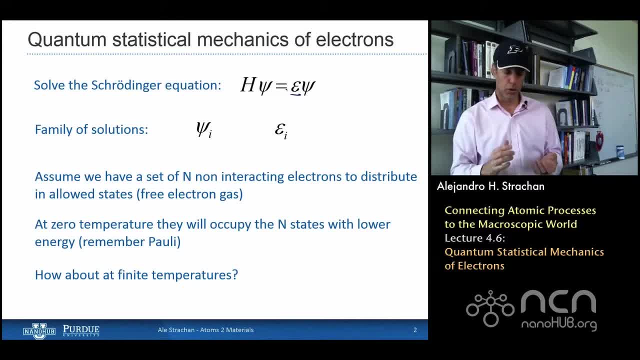 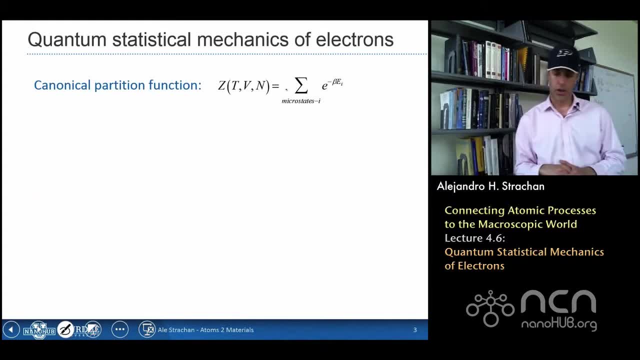 state instead of occupying the n lowest energy states. So that's what we will discuss in the lecture. now I'm going to use, as we've done in the past, the canonical ensemble, And I need to calculate the canonical partition function, If you. 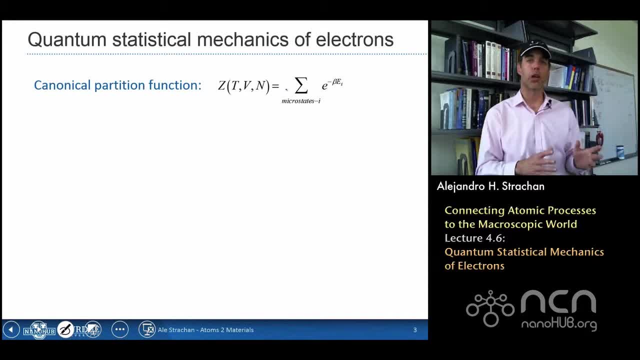 remember this involves summing over all possible microscopic states of the system of the Maxwell-Boltzmann weight e to the negative beta, the energy of that microscopic state. Okay, great. So how am I going to describe microscopic states? Well, you can see that I'm going. 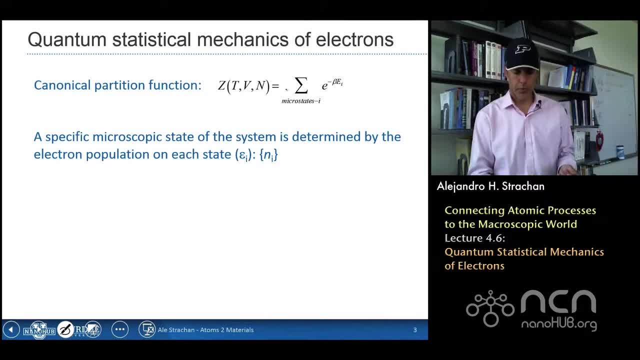 to use the mathematical formula. Well, very easily, I'm going to define a set of numbers- n sub i- that tell me the population of each of the available electronic states. So n sub i for each i can be zero if there's no electron, and it can be. 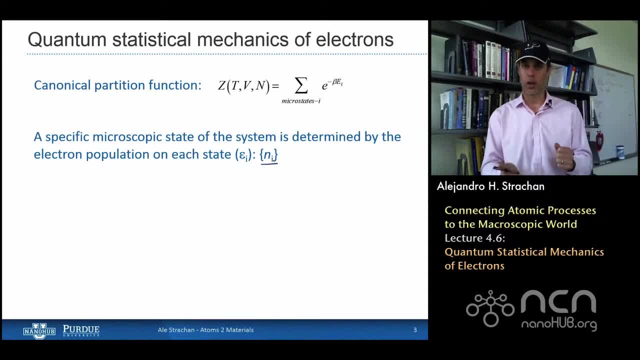 one if there's one electron in that particular state. And those are the only two options for n sub i. Okay. so the total energy of an electron is going to be the energy of the microscopic state given by a set of n sub. i's Okay, n sub 1,. 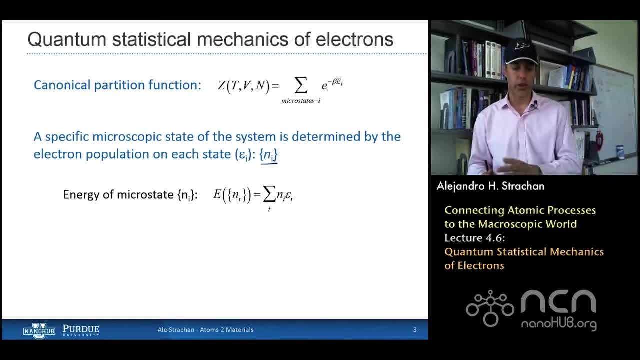 n sub 2, n sub 3 is the sum, over all of states, of the eigenvalue, the energy of that state, epsilon sub i, times the occupation, zero or one. Okay, so essentially what I'm going to do, this sum is: 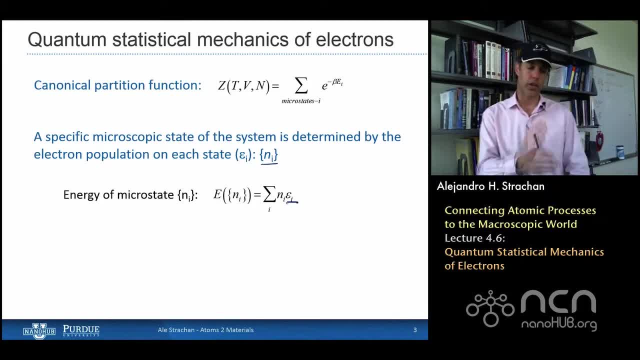 the sum over all the energies of the occupied states. Okay, that's going to be the sum over all the energies of the occupied states. Great, So now to compute the canonical partition function, what I need to do is sum over all possible states, given the number. 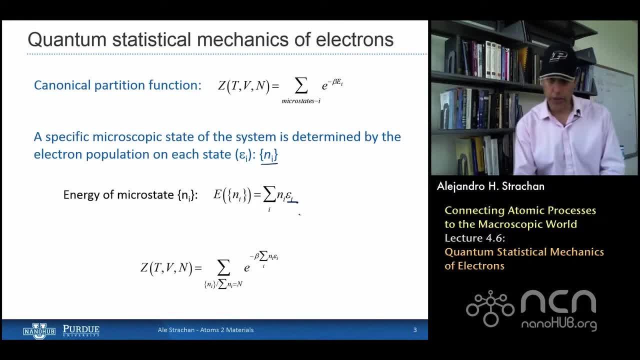 of electrons n. Okay, so I'm going to sum over all possible combinations of zero, zeros and ones such that, when I add them all up, I have my n electrons, and what I'm summing is the Maxwell-Boltzmann. 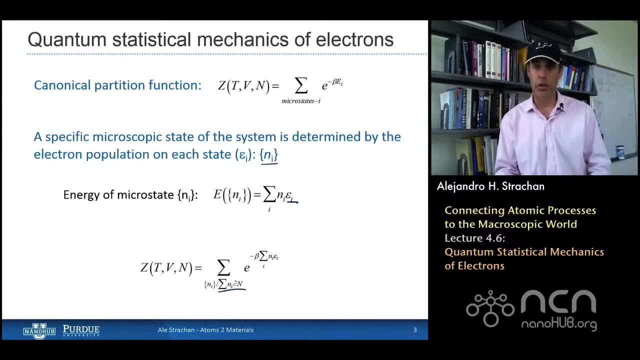 equation. Okay, so I'm going to sum over all possible combinations of zero, zeros and ones such that, when I add them all up, I have my n electrons and that's e to the negative beta, the energy of that state. 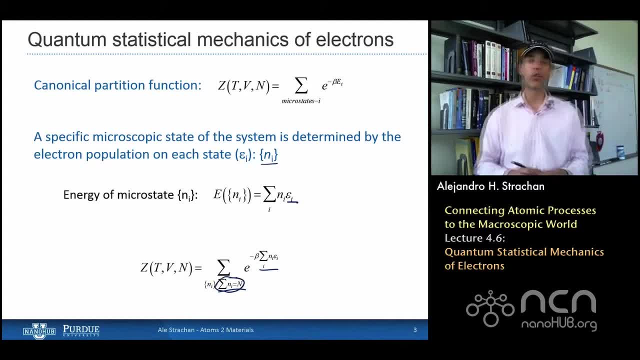 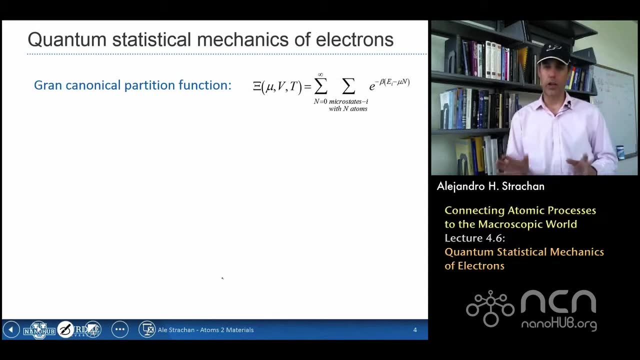 Okay. now the problem is that this constraint on the sum- the fact that I need to sum over all states such that the sum is n- makes this mathematically very complicated. Now we have a way out, because in statistical mechanics we know that we can in the 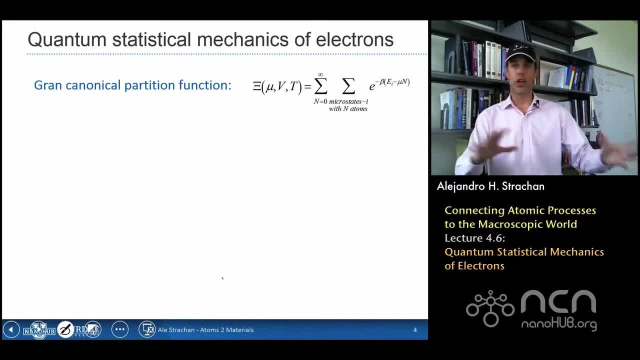 thermodynamic limit, we can change ensembles. The results of all different ensembles are consistent with one another because fluctuations are very small. So instead of using the canonical ensemble, where the number of electrons is constant, I'm going to use the grand canonical ensemble, where the number of electrons 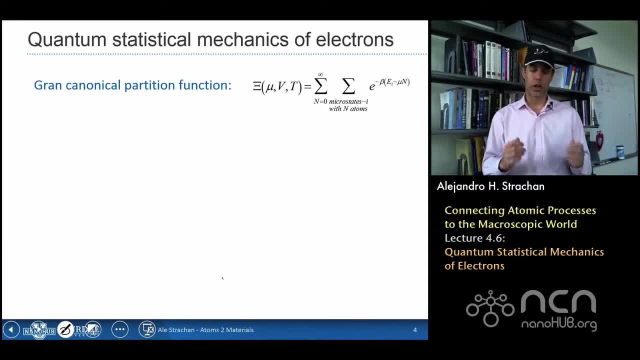 can be anything. Okay, so we're going to compute the grand canonical partition function. that involves summing over all possible states, given the number of electrons and the number of electrons in the system. So we have the principle of summing over all possible microscopic states, over all possible. 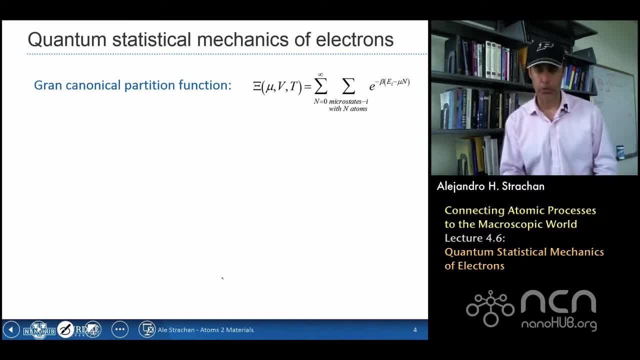 electron numbers, and then it's the Maxwell-Boltzmann weight, with the addition of the chemical potential times n. So, as a reminder, the grand canonical partition function applies to a system with permeable walls, that can exchange energy with its environment, that can also exchange particles with the. 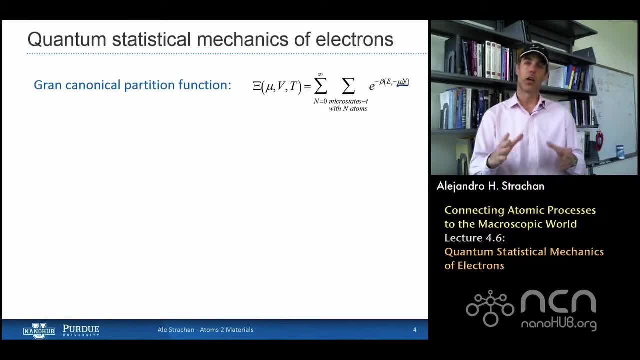 environment. So in principle, that system can be used to have zero electrons: one, two, three. the number of electrons is not a constraint. Okay, so I need to sum over all possible states without any constraint on the total number of this. 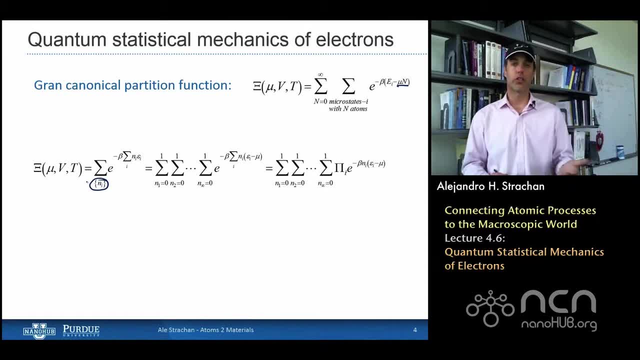 Maxwell-Boltzmann weight, which I need to modify with the chemical potential, like that. Okay, so this is the grand canonical partition function that we're going to use for the grand canonical partition function. Okay, so this is the grand canonical partition function that we're going to use for. 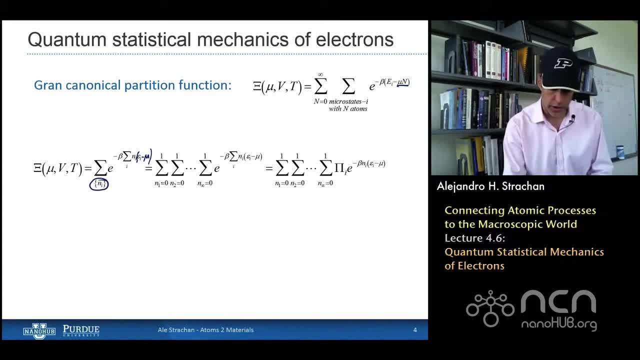 the grand canonical partition function. Okay, so this is a simpler sum, because each case for each state, individually and independently. I'm going to take the value of zero and one, So n one can be zero and one n two. the population of the second eigenvalue can be zero and. 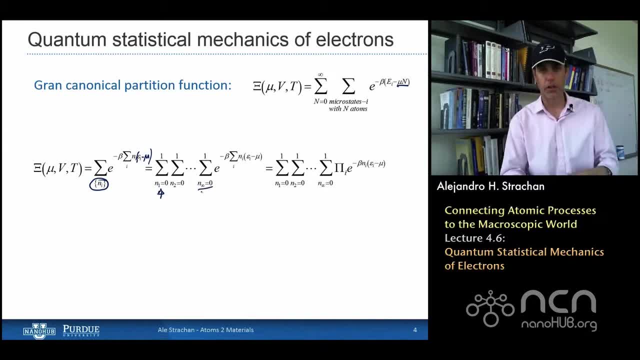 one, n, three, zero and one, all the way to infinity, if I have an infinite number of eigenvalues. Okay, and again what I'm summing here: this exponent is an additive quantity, because my electrons are non-interacting, and the exponential of a 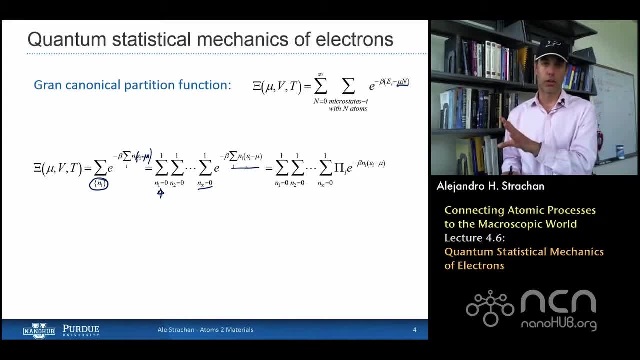 sum is the product of exponentials, so I can write the sum in this way. Now I can switch the order between the product and the sums- okay, and I end up with a product over all of states. okay, and I can write the product over all of states. 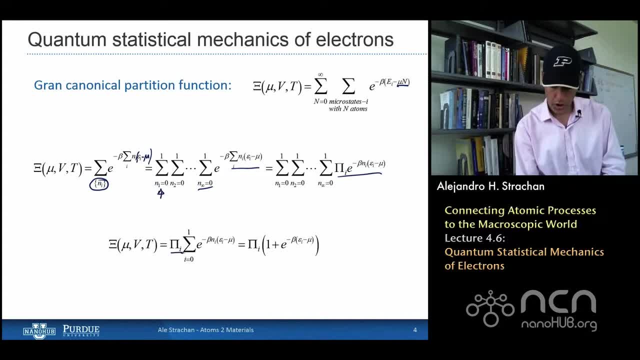 okay, and I can write the product over all of states. okay, and I can write the sum of the sum of the possible population of that state. Now, the possible populations of a given state are only two, zero or one, and so it's the product of over all. 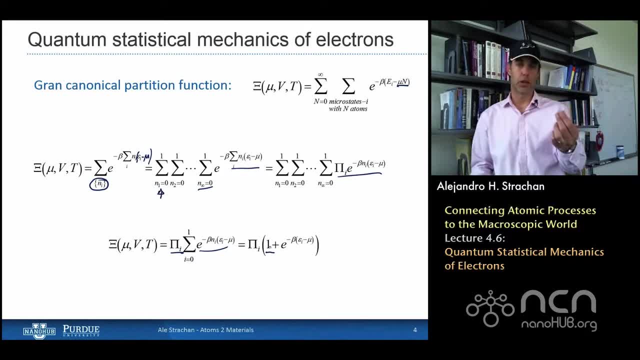 of states of one, that's the Boltzmann weight when there's no electrons in the state, plus e to the negative beta, the energy of the state minus the chemical potential. Okay, so by lifting the restriction of the number of atoms, switching to the grand canonical ensemble, I. 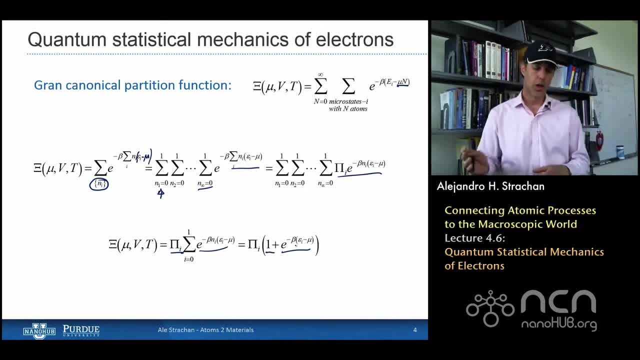 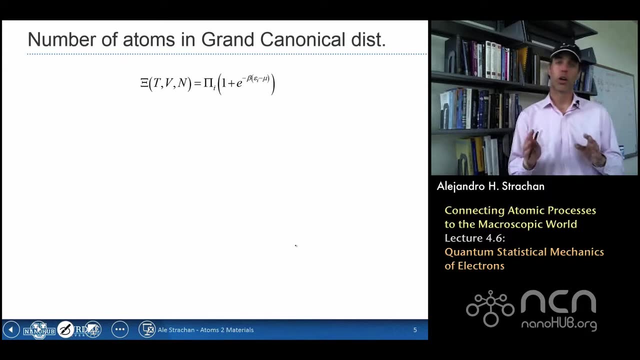 can then solve the partition function for a system given a chemical potential and a temperature of the heat bath. okay, So that's where we are. I have an analytical expression only because I have non-interacting atoms and with this analytical expression, with the 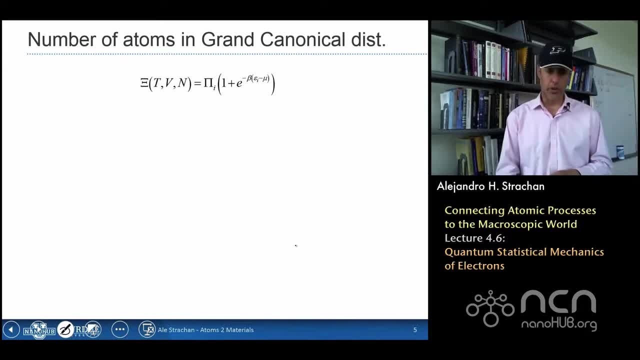 potential of the heat bath. okay, so that's where we are. I have an analytical expression for the partition function, If you remember from two lectures ago. we can compute the average number of atoms n for that chemical potential and temperature as the derivative of 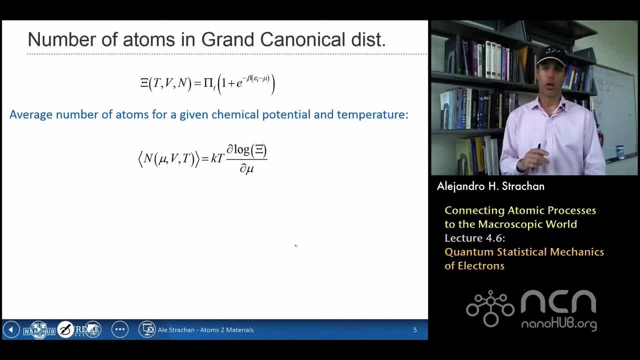 the log of the partition function with respect to the chemical potential mu, and I can do that very easily. okay, the grand partition function is the product, so the log is the sum, and then you just have the contribution of each state of the particle, and then 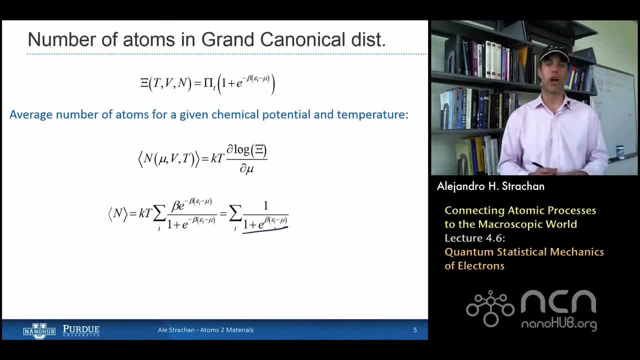 you can assign a specific state to the average number of atoms. okay, so the average number of atoms is the sum over all possible states of this little contribution and of course you can immediately assign a meaning to that contribution. that's the average occupation of that particular. 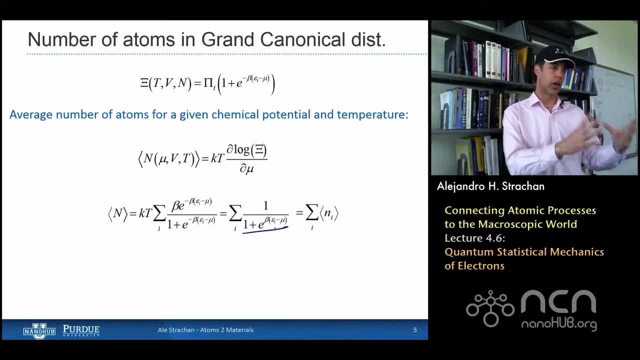 state: okay, so the total number, the average number of electrons, is the sum over states of the average number of electrons in that particular state, and then you can immediately calculate the number of electrons in that particular state, and that is called what we just found. 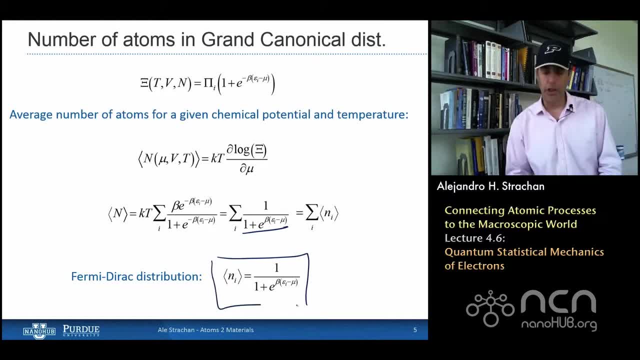 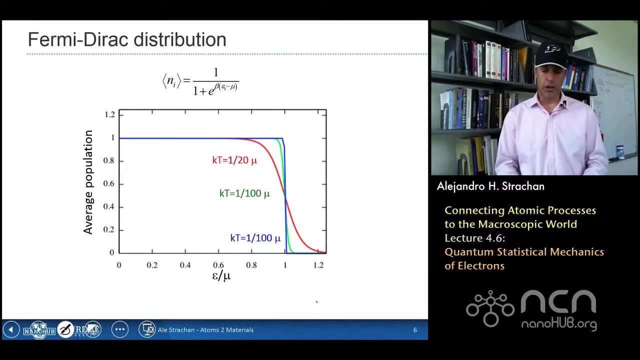 is the Fermi Dirac distribution. okay, so the Fermi Dirac distribution gives us the average population of a state of energy epsilon i at the given temperature and chemical potential. So let's look at this distribution a little bit. what I'm doing here is plotting the 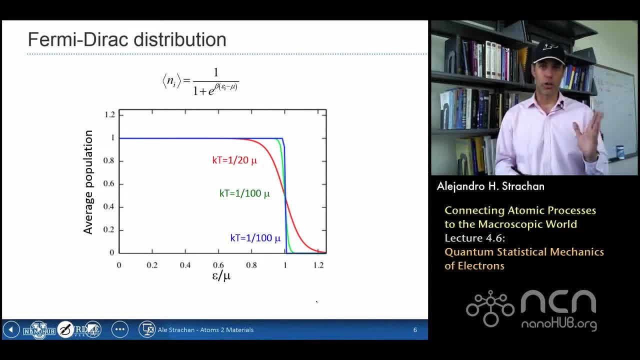 distribution for three different temperatures. let's start with the lowest temperature, and then there's a typo here. this is the chemical potential, over 1,000, so very, very small temperature, and what we find is that the Fermi Dirac distribution is essentially one. so 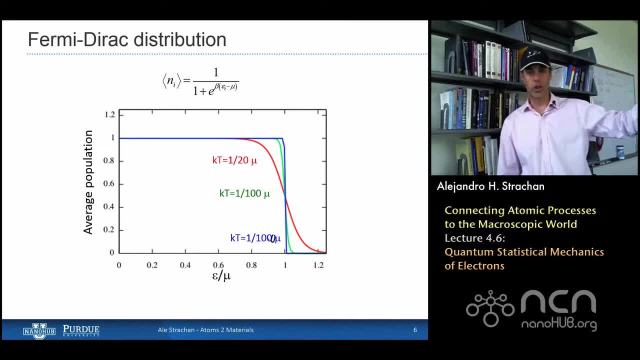 the average number of electrons per state is one, up to the point where of the chemical potential. okay, so this value here is the chemical potential, also called the Fermi energy. So this is the Fermi Dirac distribution, the Fermi energy. so the states, all the. 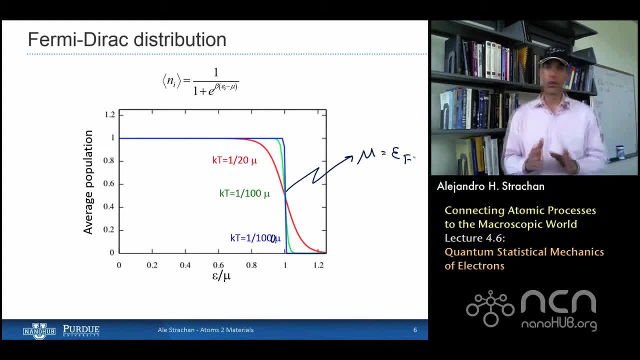 states with energy less than the chemical potential are occupied. all the states with energy higher than the chemical potential are unoccupied. okay, If I increase the temperature a little bit, crank up the temperature a bit to the chemical potential over 100, then we go to. 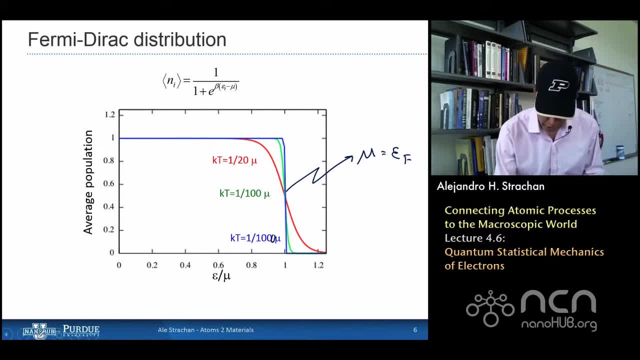 the green curve and you can see here in the green curve that I have promoted some electrons to the green curve and then the electrons that were right below the Fermi energy to an unoccupied state, right above the Fermi energy. okay, Remember, this function tells: 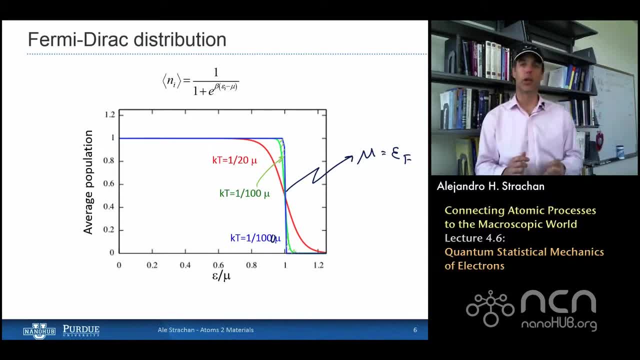 me the average number of electrons. so if the average number is a little bit less than one, that means that those atoms- I'm sorry, those electrons- have been promoted. they're going to spend some time at the higher energy state, If I increase the temperature even. 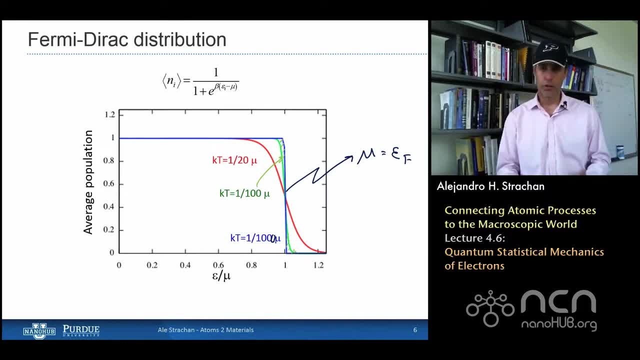 higher. I increase the temperature even higher, even more. seeing the red curve that the amount of excitation is bigger, I go deeper in energies to dig up electrons and move them up to unoccupied states. Now here the Fermi, the Pauli statistics, the Pauli exclusion. 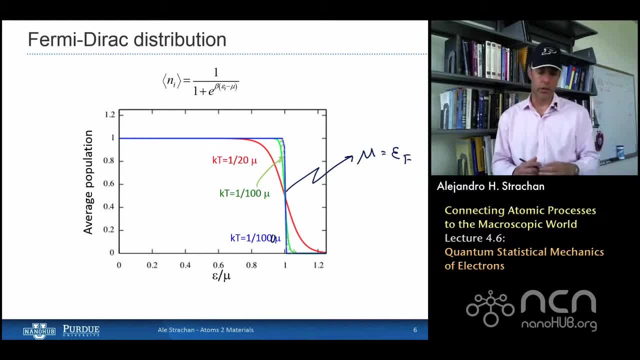 principle plays a key role. So these low energy states, even though I'm at a high temperature, nothing can happen unless I increase the temperature a little bit to unoccupied states, Even though I'm at a high temperature, nothing can happen to them. Those electrons, 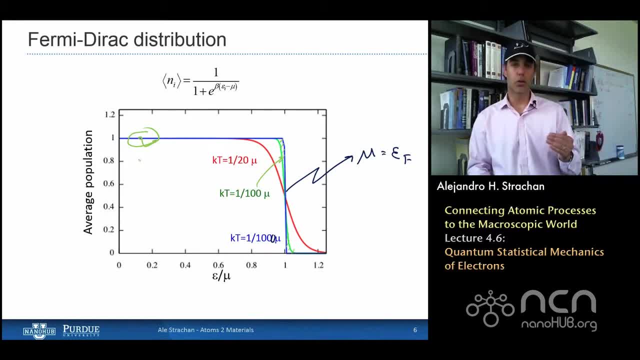 that are down here cannot be promoted because there's no. even though there's quite a bit of energy in the system, there's no empty states for these electrons to be promoted. So all the action happens near the Fermi energy or the chemical potential of the system. So 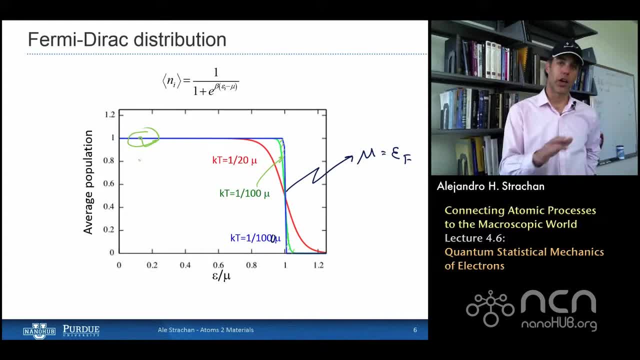 if you have taken some of the prior courses in nanoHAV-U on electron transport or thermal transport in general, you would be familiar with this Fermi direct distribution, and what we have done in atoms to material is learn how it originates from fundamental physics. 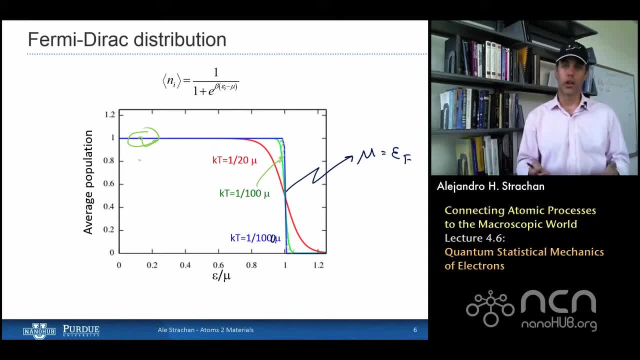 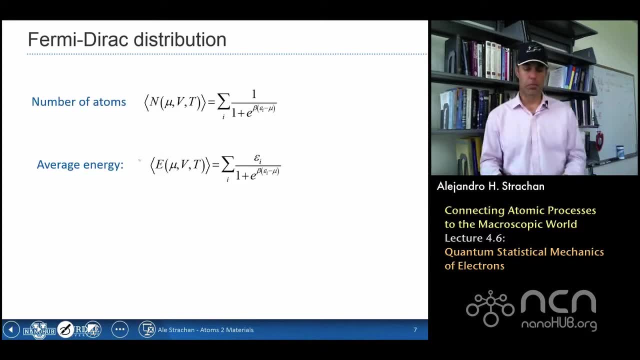 Now. so just to sum up, we've computed the average energy, the average number of electrons in the system and the average number of electrons in the system, and the average number of electrons in the system and the average number of electrons in the system. That's just. 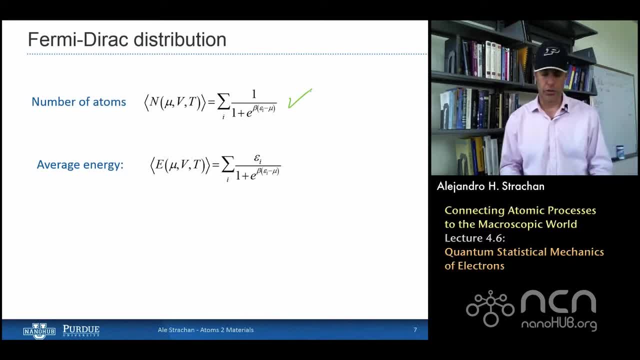 the sum over all eigenstates of the Fermi direct distribution. I can compute the average energy in the system in a very similar way by summing over all possible states, all eigenstates of the average number of electrons in that state times their energy. So we can rewrite this: 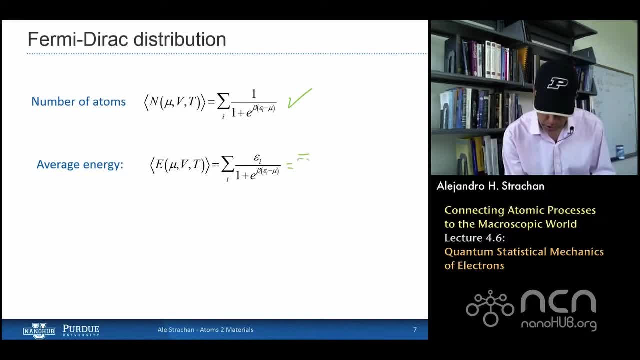 as the sum over states of energy. epsilon sub i times the energy. and then we can compute the sum over states of energy- epsilon sub i times the average number of electrons in that state and compute the energies that way. Now one theory that we're not going to. 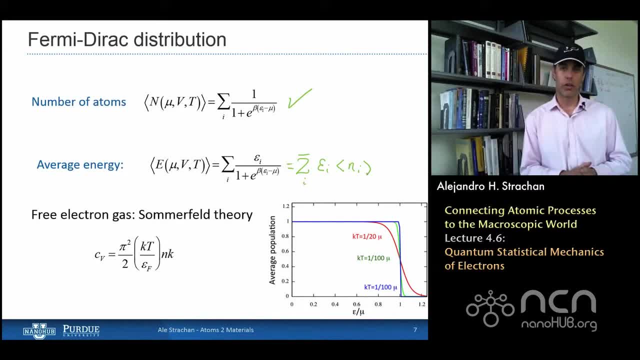 have a lot of time to discuss in detail is the Sommerfeld theory of metals. So Sommerfeld described metals in a very, very simple way. He assumed that the number of electrons in the system is equal to the number of electrons in the system and the number of 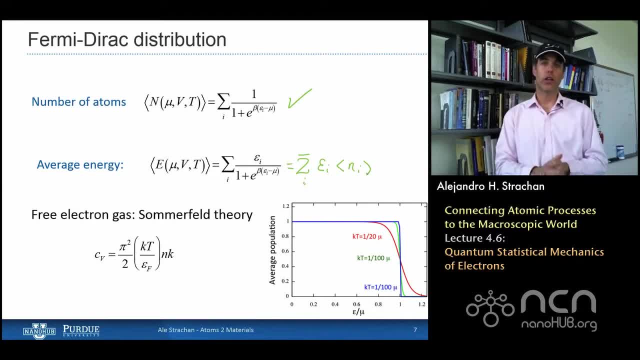 electrons in the system is equal to the number of electrons in the system. So he found that the electrons were a set of non-interacting particles that lived in a flat potential and very much like what we did, exactly like what we did with the electron in the box. 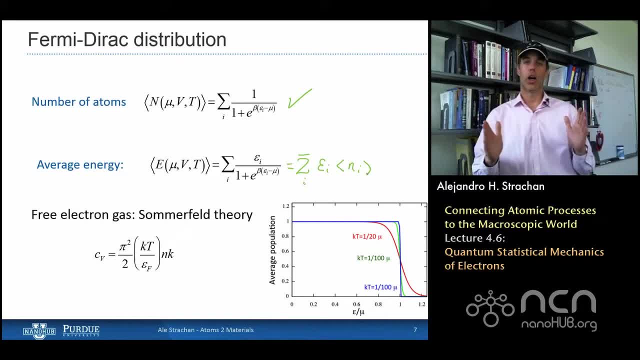 in weeks one and two. So he did the same approximation. he made the approximation that the electrons didn't interact with one another and he solved the statistical mechanics of the electrons in this manner, And one of the things that you can predict using this. 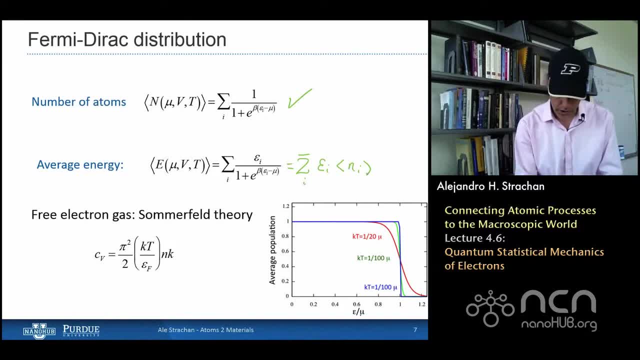 Sommerfeld theory is that the specific heat of electrons at low temperatures is proportional to temperature, So the electronic specific heat goes to zero in a way that's proportional to temperature. And this is a huge success of the Sommerfeld theory, even though it's a little bit more complicated. 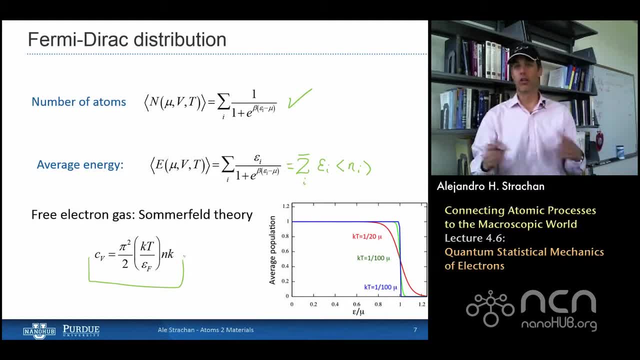 than what we're used to, but it's still very interesting. He made all these approximations that the electrons don't interact, that they live in a flat potential, and still was able to capture some of these very interesting physics that you see experimentally. So this implies: 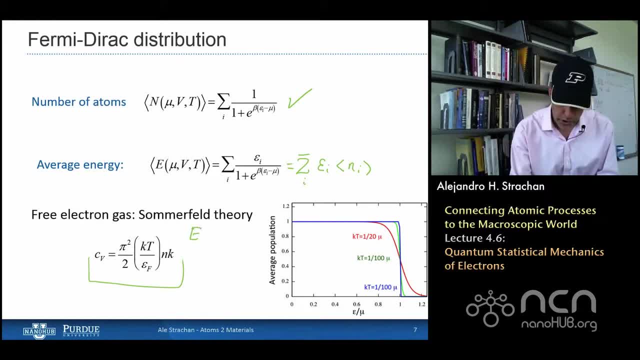 the specific heat being proportional to kT implies that the energy is proportional to kT squared, And while we're not going to derive the Sommerfeld theory, we're going to use the course. we don't have time for it. it's relatively easy to understand why the energy 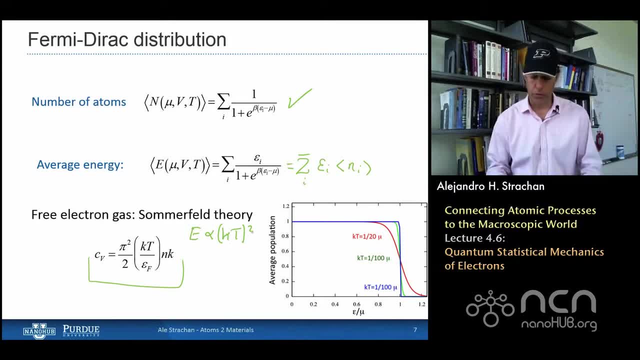 is proportional to t squared. If you look at the Maxwell-Boltzmann, at the Fermi-Dirac distribution, the amount of excitation, the depth of the number of electrons that get promoted, is proportional to kT. So if I have kT of 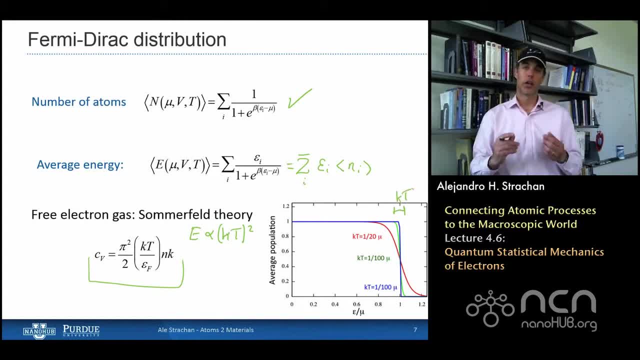 thermal energy electrons that are at low temperatures are proportional to kT squared. So if I have thermal energy, electrons that are within kT of the Fermi energy are going to be promoted. Of course, the average energy of those electrons, of each one of 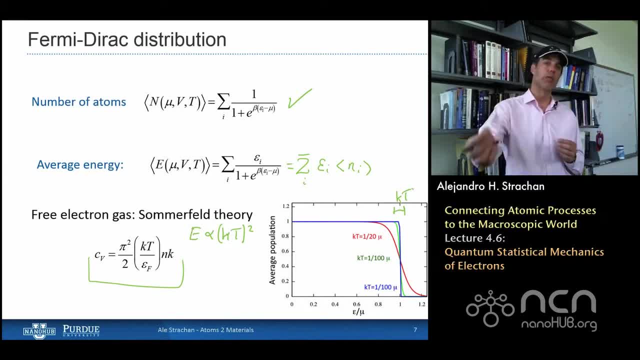 those electrons is also approximately kT, the average extra energy, how much they move, And so I have kT electrons with kT energy. the total energy, thermal energy, in the system is kT squared, and that leads to the specific 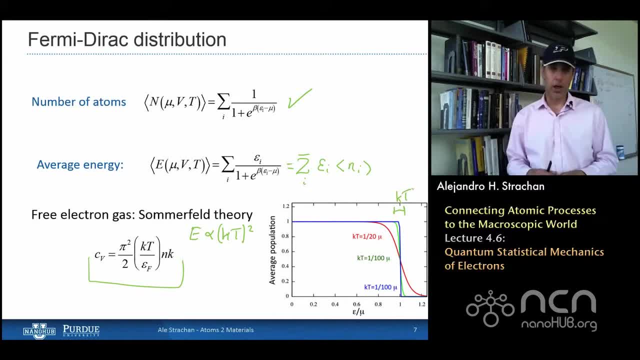 heat being proportional to temperature. If you'd like to read more about the Sommerfeld theory of metals, you can consult any solid state physics book like Ashcroft-Merman. and what we have done in Atoms to Materials is give you the fundamental understanding that 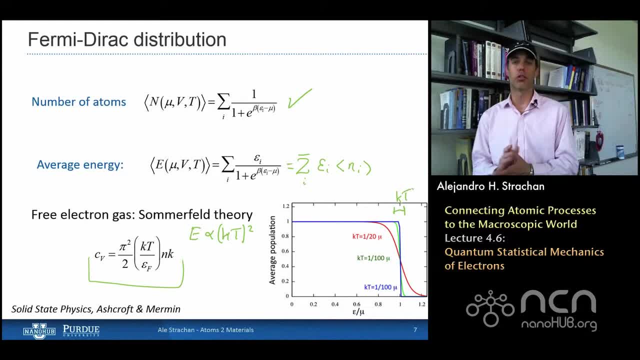 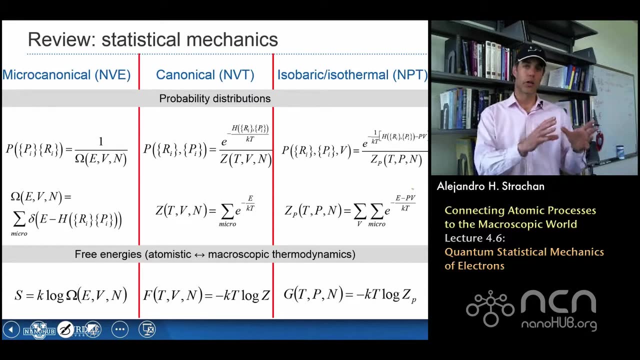 would allow you to read and learn about the Sommerfeld theory without much trouble. So just to sum up a little bit, what we're going to do is we're going to use the results. What we have done during this week is connect the microscopic worlds, microscopic and. 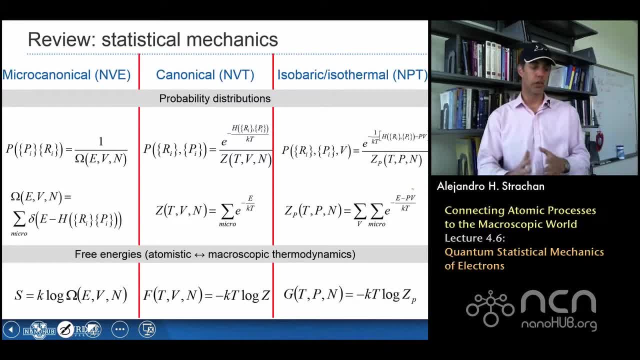 microscopic worlds back and forth. And if you go back through the lectures you will notice that the only assumption that we made was done very early on in the first lecture where we said that for an isolated system in the microcanonical ensemble, all the microscopic 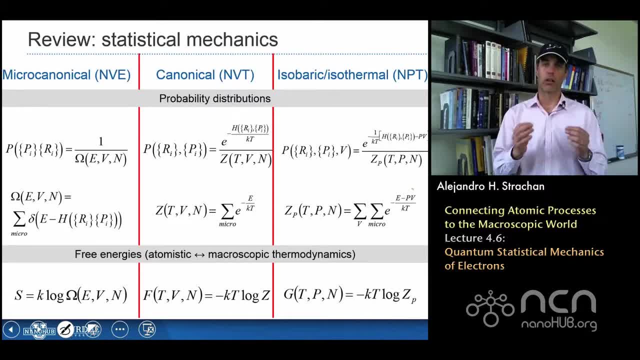 states were equally likely, of course. So that's what we're going to do. So the equal a priori probability postulate was the only assumption we made. All the rest was derived, and we're very successful at reconstructing thermodynamics and understanding the connections. 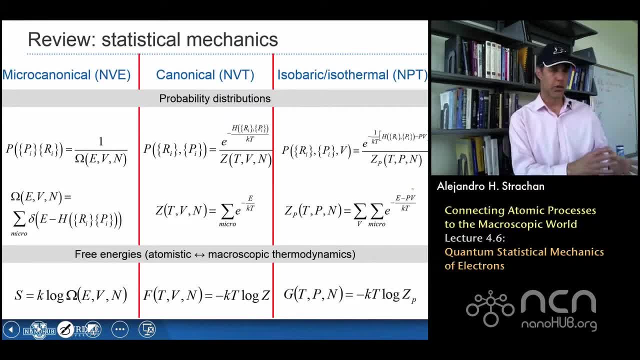 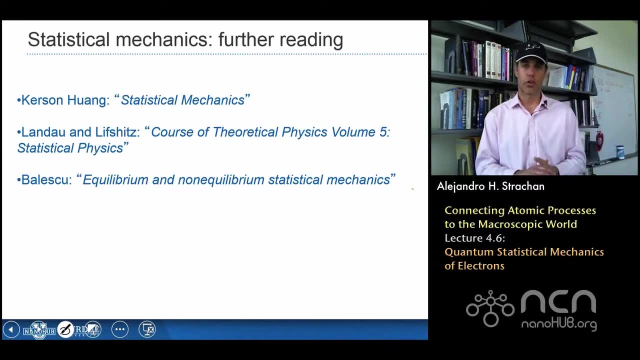 between electronic and atomic processes and thermodynamics. So of course statistical mechanics is a very broad and deep field and we can only scratch the surface of the thermodynamics. and we can only scratch the surface of the thermodynamics and we can only scratch the surface in a week. But hopefully what you learn 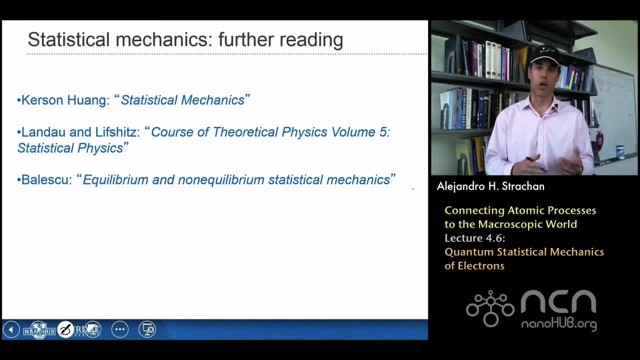 in atoms to material will motivate you to read more and learn more about statistical mechanics, and, if not, at least when you read a paper that uses statistical mechanics, you would understand the origin of the assumptions that they make or the origins of the equations that you encounter. So with that I'll end. 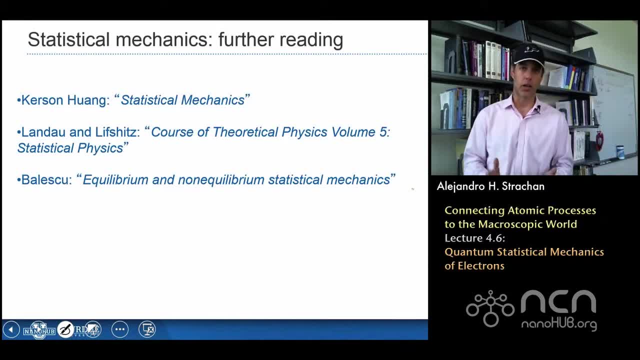 and I'll see you all in the next lecture. Thank you very much. 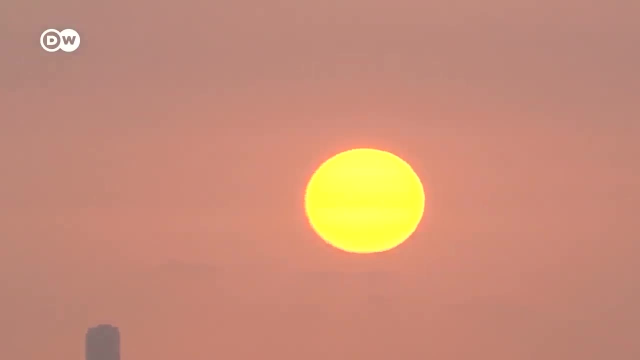 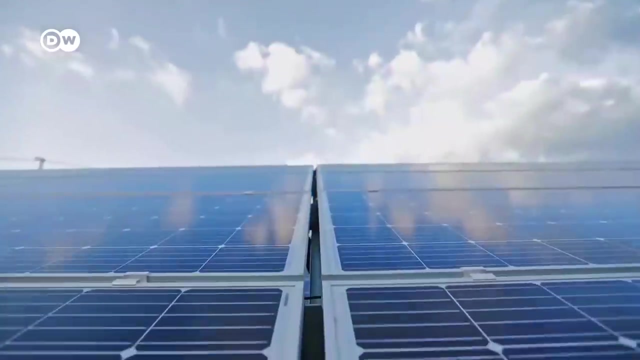 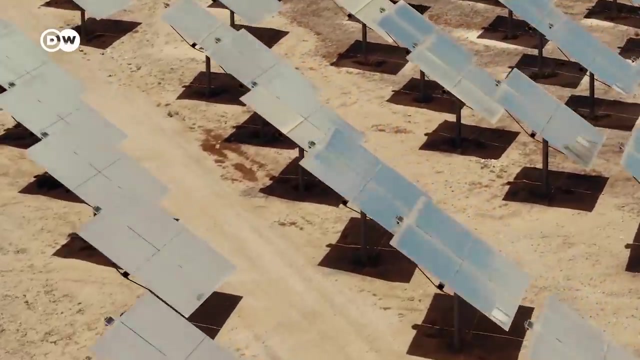 It's astonishing, but clean energy from the sun, solar energy, has become the cheapest way to generate electricity. It's even cheaper than coal, And yet it produces only 3% of the world's electricity. Why aren't we using way way more of it?